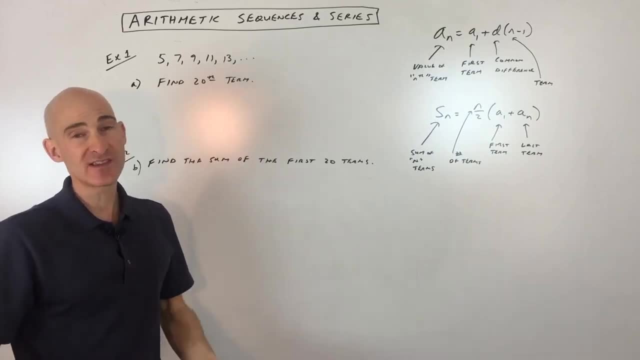 In this lesson we're going to talk about arithmetic sequences and series. So what's an arithmetic sequence and what's an arithmetic series? Well, sequence just means that it's a list, And what makes it arithmetic is that you're adding the same thing each time to get to the next. 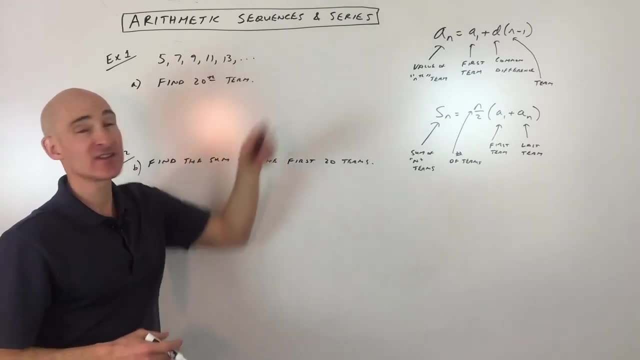 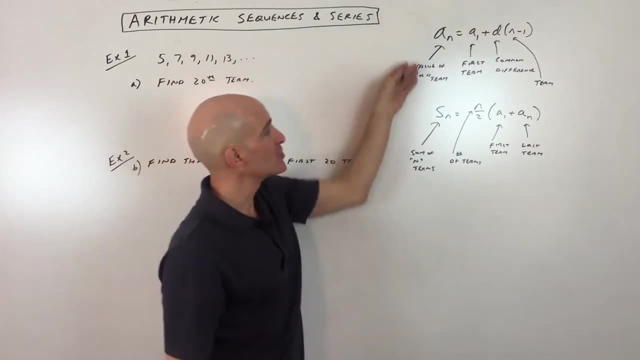 term, the next term, the next term And then a series is basically a sum. It means that you're adding up all those terms in that arithmetic list, that arithmetic sequence. So a couple formulas that are good to know and memorize are the formula that allows you to find the nth term. 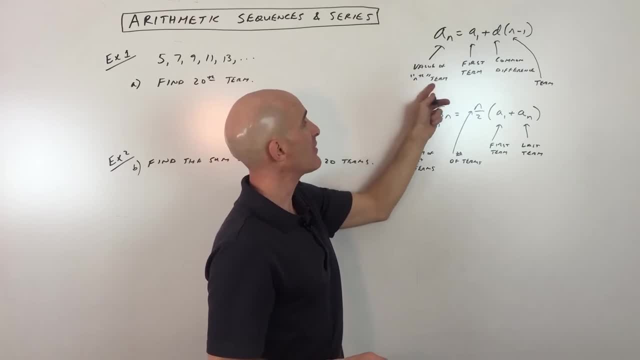 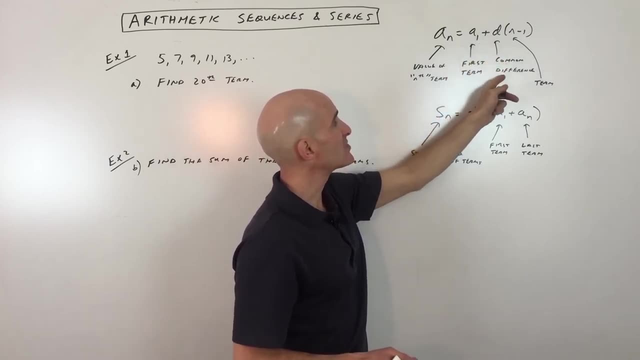 And what this tells you is that a sub n is the value of the nth term and it equals the first term, which is a sub 1.. So 1 just means the value of the first term plus d, which is the common. 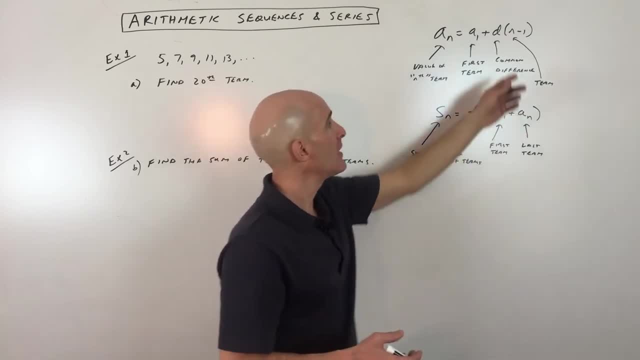 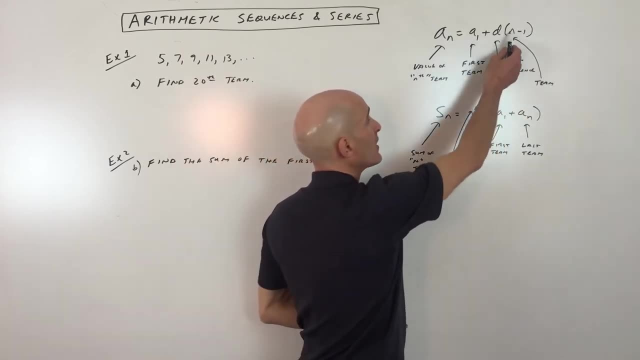 difference. That's what you're adding or subtracting to get to the next term, And then times the quantity n minus 1.. And n just refers to whatever term that you want to find. If it's a hundredth term, then n would be 100.. a sub 100 would be the value of that hundredth term. And then this: 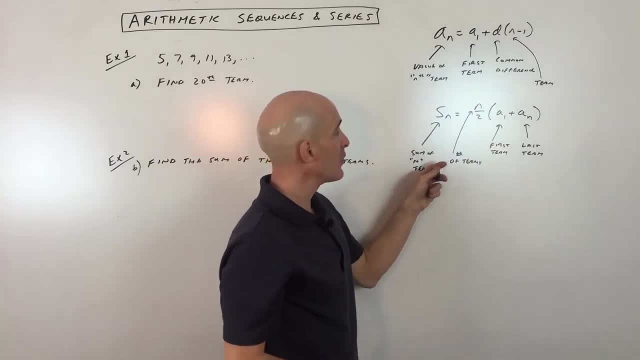 formula here which is the sum of n terms. which means, if you're just, you know, adding up, you know n terms. you would take the number of terms, n. So if there's 20 terms, it would be 20 divided by 2.. And then you take the quantity of the first term. 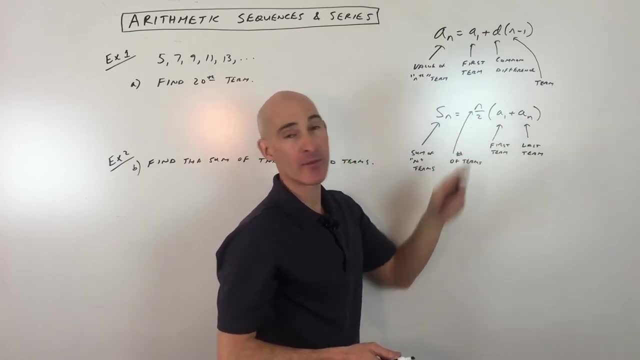 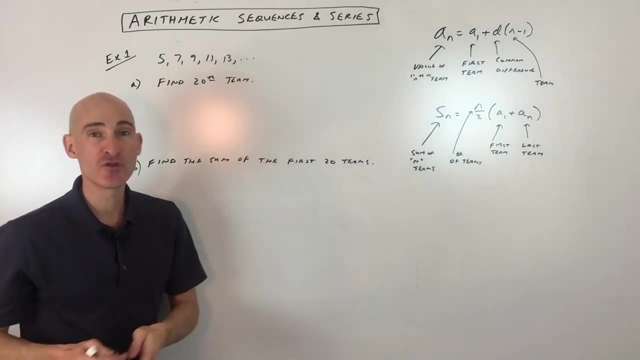 you know, plus the last term, So that quantity added together multiplied by n over 2.. So let's go through a couple of examples. Go ahead and pause the video, See if you can do these on your own. I hope that this is familiar to you from your Algebra 2 class, But if not, we can review it here. 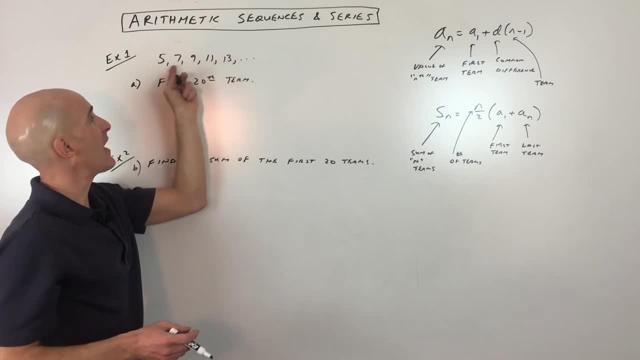 So they're giving us the sequence, this list. here It's 5,, 7,, 9,, 11,, 13,. dot, dot, dot and so on, And it's like a two-part question. One, it says: find the 20th term Okay. And then part two says you. 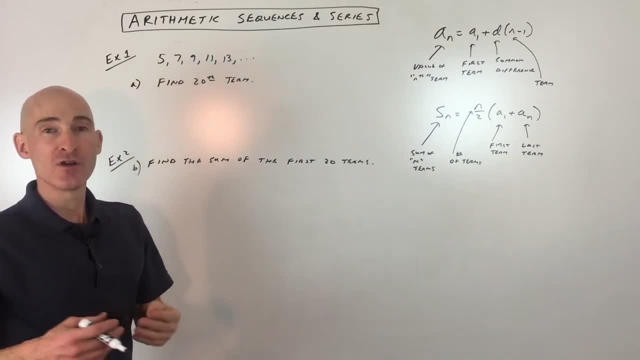 know, find the sum of the first 20 terms. Well, go ahead and see if you can do this on your own. We'll do it together, But there's not that many terms- 20 terms. if you wanted to, you could just. 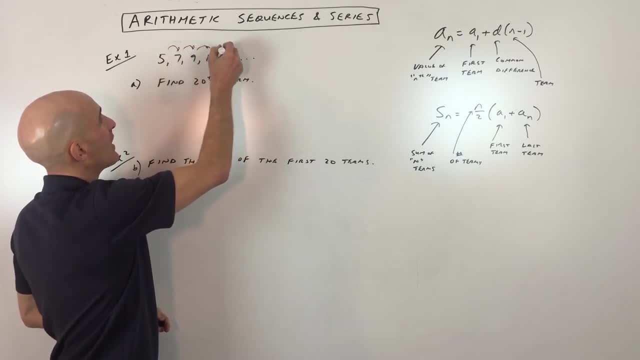 keep. you can see they're adding 2 each time. You could just keep adding 2,, adding 2,, adding 2.. And you could write those out. It's not that many. You could then, you know, go ahead and find that. 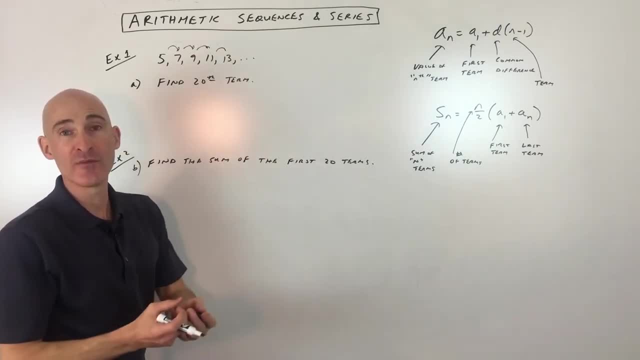 20th term, And then the sum. you could then go ahead and you know, add all of them up. So it would be a way of understanding that you know this pattern continues. You keep adding 2. That's.